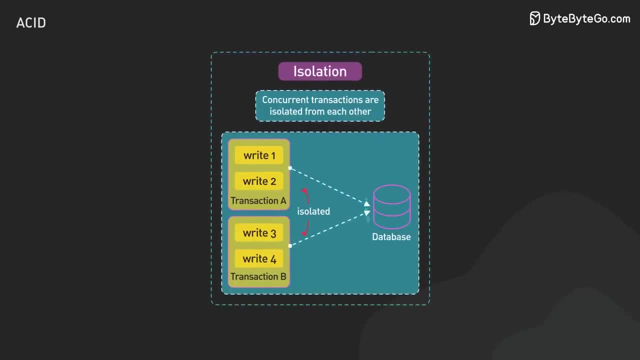 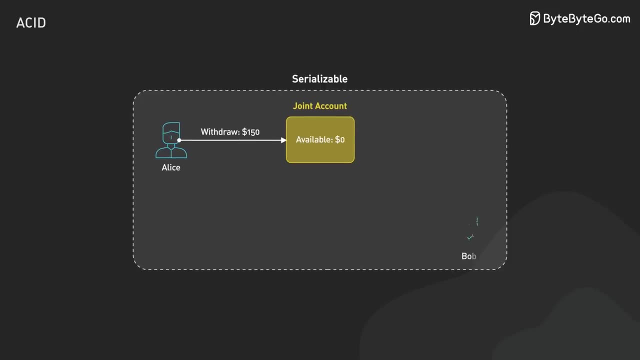 Even if many transactions are running at the same time, isolation makes it seem like each transaction has the database all to itself. The highest level of isolation is called serializable. It makes transactions run very fast. It makes transactions run very fast. It makes transactions run very fast. 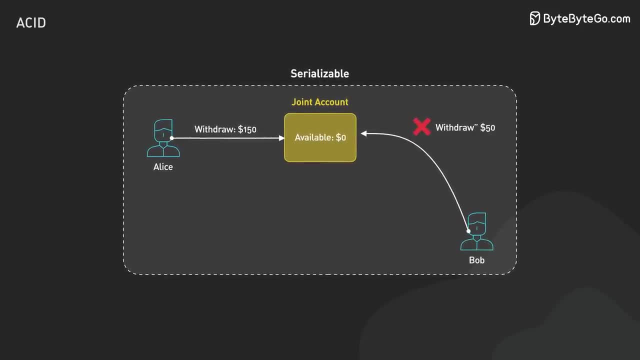 It makes transactions run one after another as if they were in a single line. This provides the strongest consistency, but it can really slow things down because each transaction has to wait its turn. To speed things up, databases often provide lower isolation levels that allow more transactions. 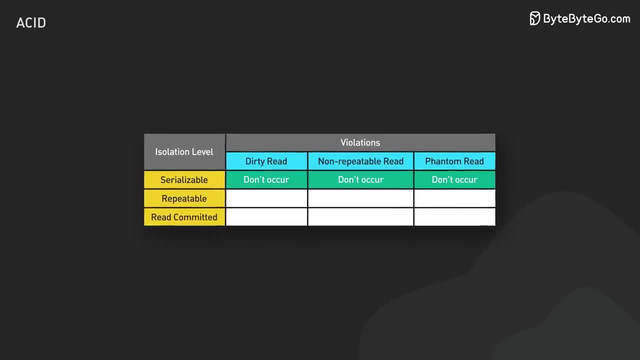 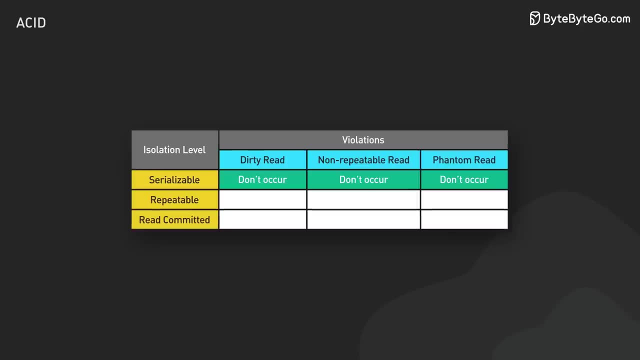 to run simultaneously. But there's a catch. These lower levels can sometimes lead to inconsistencies like dirty reads, non-repeatable reads and phantom reads. A dirty read happens when a transaction sees data that was changed by another transaction that hasn't been committed yet. 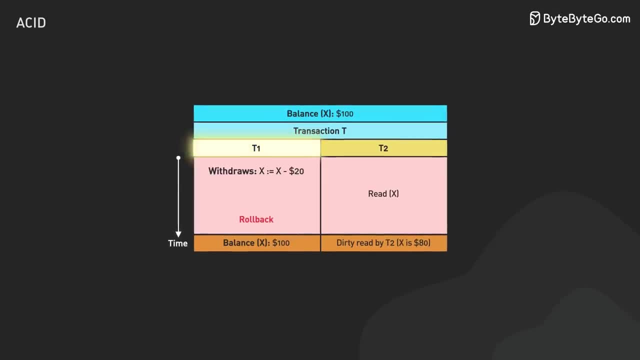 Imagine a bank account with $100.. Transaction T1 withdraws $20 but doesn't commit. If transaction T2 reads the balance before T1 commits, it will see $80. But if T1 rolls back the $80 balance never truly existed. 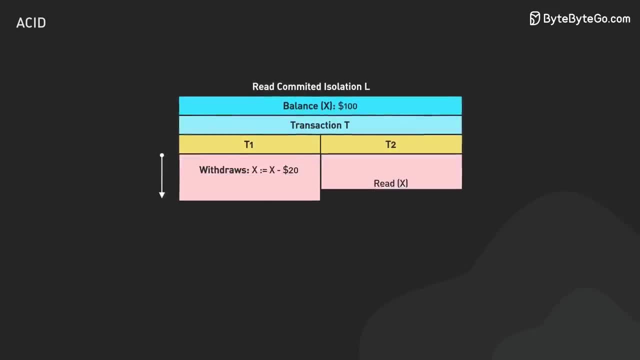 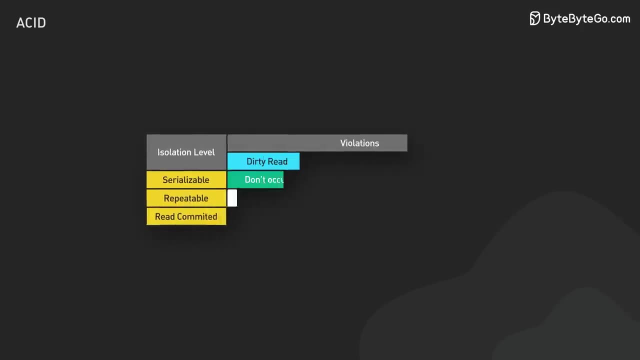 It's a dirty read. The read-committed isolation level prevents dirty reads by making sure a transaction can only see committed data, But you can still have non-repeatable reads. Where a transaction reads data, it's not a non-repeatable read. 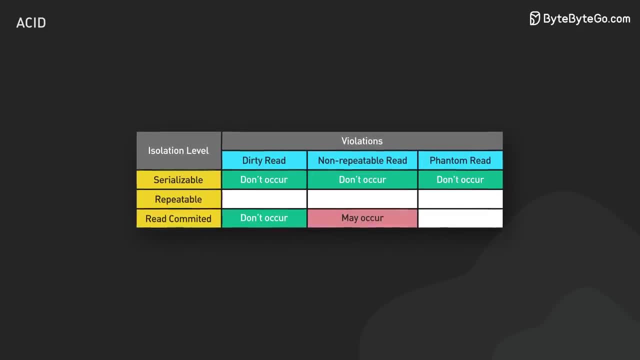 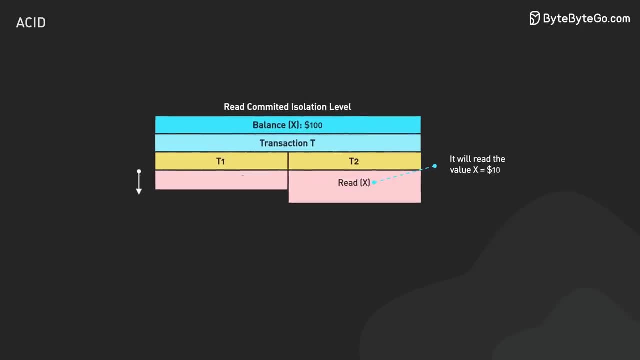 It reads the same data twice and gets different results because another transaction changed the data in between. For example, say you check your bank balance and see $100. Then another transaction withdraws $20 and commits. If you check your balance again in the same transaction, you will see $80. 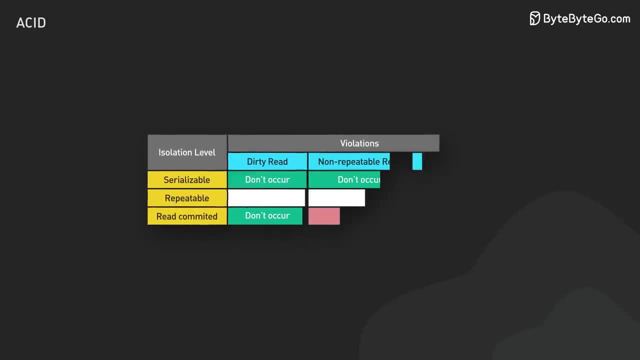 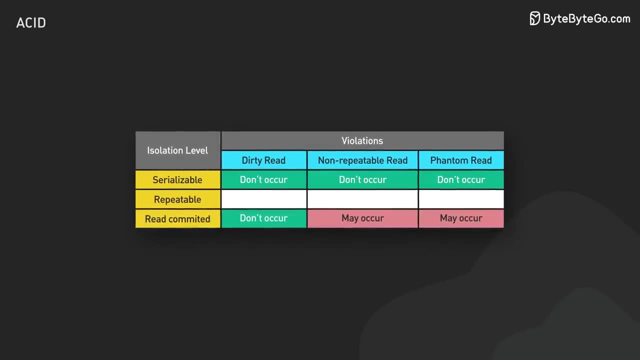 That's non-repeatable read. Read-committed can also have phantom reads, where a transaction re-runs a query and gets different results because another transaction added or deleted rows that match the search criteria. Imagine a transaction that lists all bank transfers under $100.. 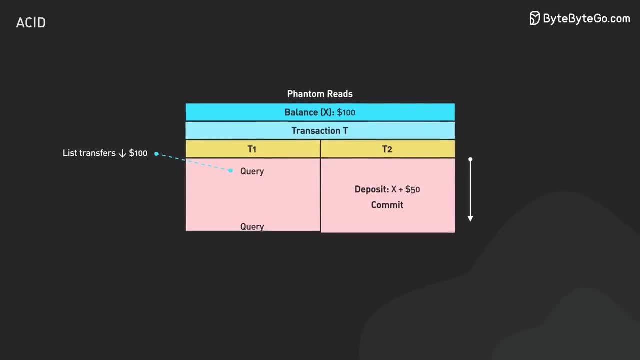 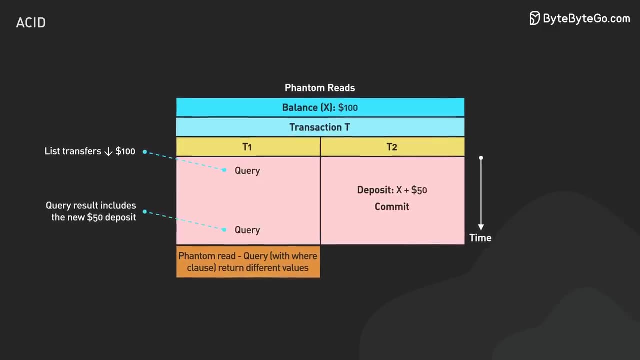 Meanwhile, another transaction added a $50 transfer and commits. If the first transaction re-runs its query, it will see the $50 transfer that wasn't there before. a phantom read. The repeatable read isolation level prevents non-repeatable reads by giving each transaction.